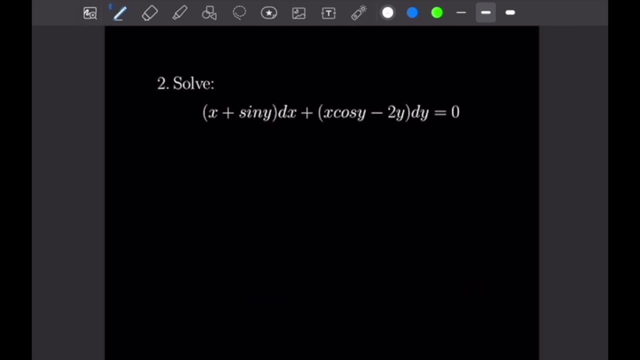 solution process for these types of problems. So, looking at this first problem, we have x plus sine y, dx plus x cosine y minus 2y, dy is equal to zero. So let's go ahead and mark out: this first part is going to be our m and this second part is going to be our n. So let's go ahead and check to. 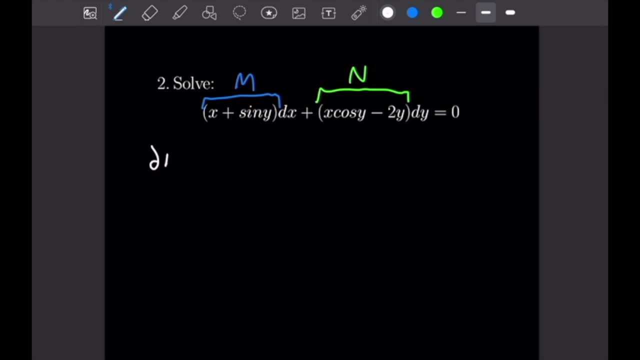 see if this equation is in fact exact. So the partial with respect to y of n is going to be, that x term is going to go away, and then we'll be left with cosine of y and the partial with respect to x of n. Let's see what we're going to get there. Well, that x is going to disappear. on that. 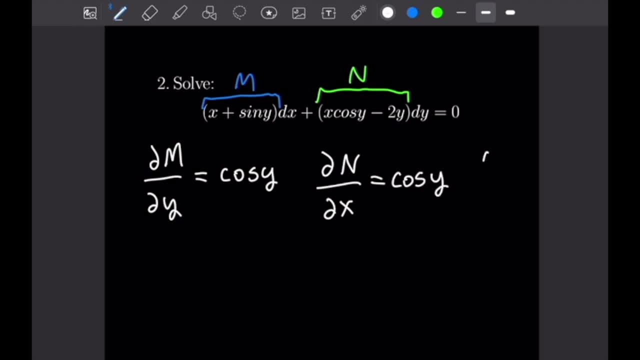 first term. so we'll just have cosine y, and that second term is going to disappear. so we can see that this equation is in fact exact. Now, to solve this exact equation, we are going to be looking for a function g of xy that satisfies the following. So by exactness, 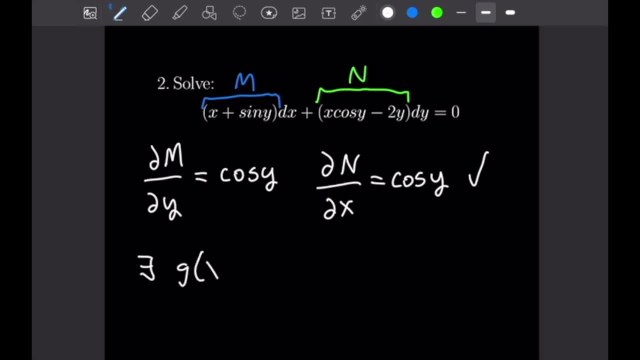 we know that this function exists. So there exists a g of xy, such that d g of xy is equal to the sum of our m and n. so we have m of x, y, dx, plus n of xy, dy, And by exactness also. 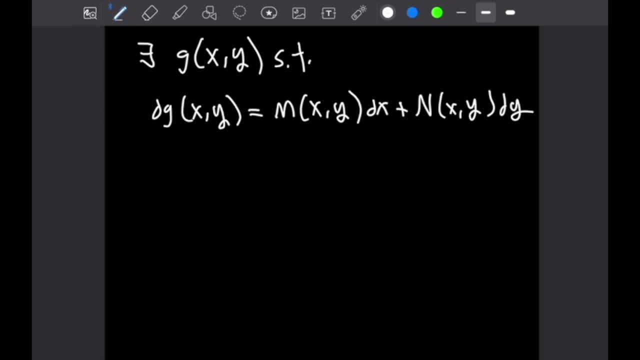 this g of xy must also follow the following two equations We have: the partial of g of xy with respect to x is equal to m of xy, and the partial of g of xy with respect to y is equal to m. So for this, therefore, 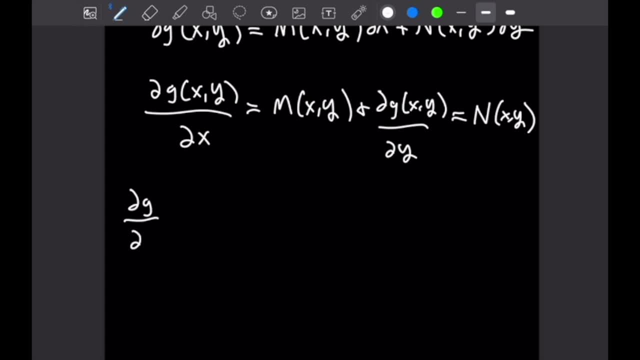 So for this, therefore, particular equation, we'll have that dg dx is equal to x plus sine y and dg dy is equal to x cosine y minus 2y. now, usually, from here we will choose which of these two equations is easier to integrate, with respect to x and y respectively. now, looking, this is going to be easier to integrate. 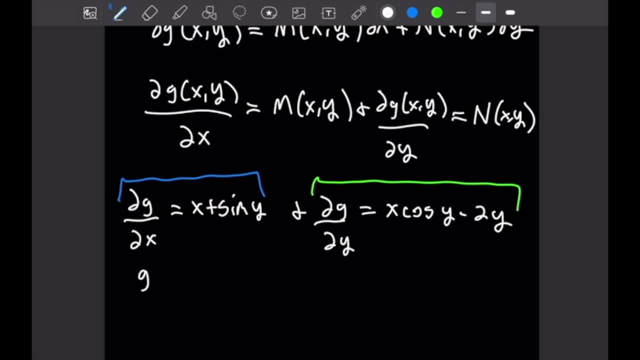 this first one. so taking the antiderivative of both sides, here we will get that g of x, y is equal to x squared over 2 plus x times sine y plus h of y, just some unknown function of y. we're going to go ahead and solve for that h of y. we're going to do that by differentiating. 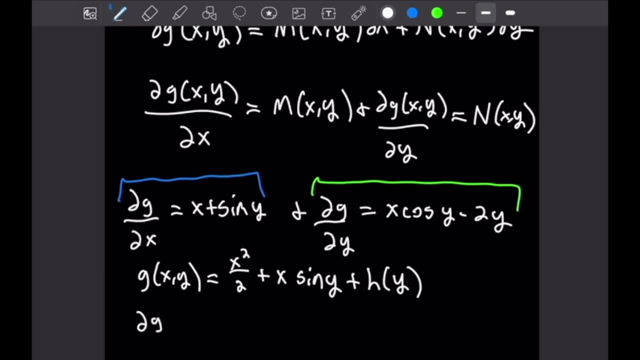 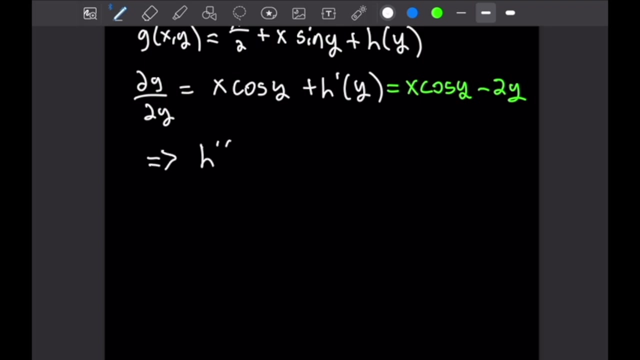 both sides. so if we do that, we'll get that d, g, d, y is equal to x times the cosine of y plus h prime of y, and we can relate this to our equation in green right here. so we can see that that is equal to x cosine y minus 2y, and this of course means that h prime of y is equal to: 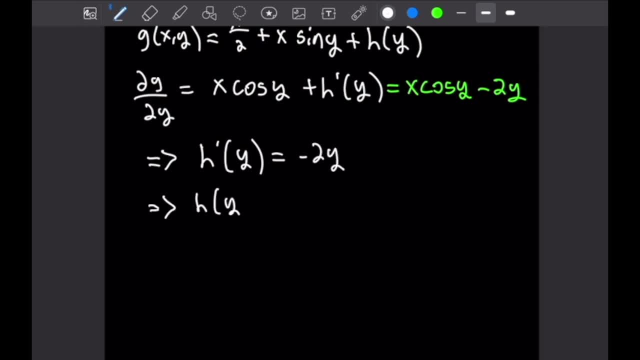 negative 2y, which means that h of y is equal to negative y squared plus some constant c and plugging that back into our original equation, we will have our final implicit solution for this differential equation. we have that g of x- y is equal to x squared over 2 plus x. sine of y minus y. 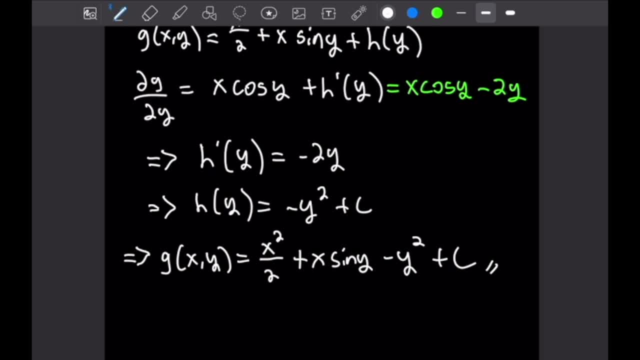 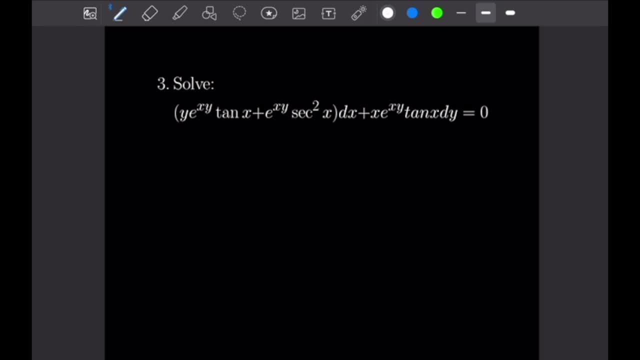 squared plus some constant c, which finishes this problem off. so let's go ahead and get to our next example. okay, so looking at number three, it says that y times e to the x y times tangent of x plus e to the x- y times secant squared of x, dx plus x times e to the x- y tangent of x- dy is equal to 0.. 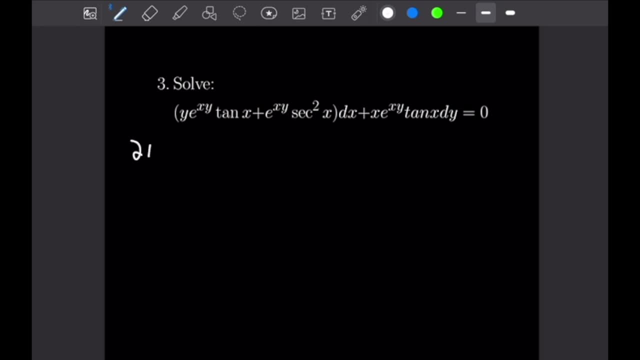 so let's go ahead and check this equation for exactness. We're going to take the partial of m, and our m is this first one here in blue and our n is this one in green here. so the partial of m with respect to y. let's see what that's going to be. well, we're. 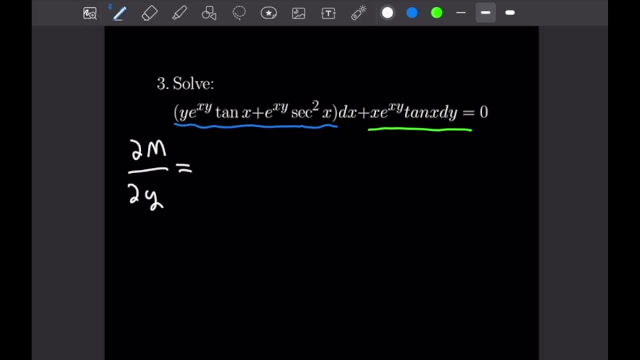 going to have to use the product rule here, so we'll have y times the derivative of e to the x- y, and that's going to be x times e to the x, y times the tangent of x and that's going to be plus e to the x, y times the tangent of x. 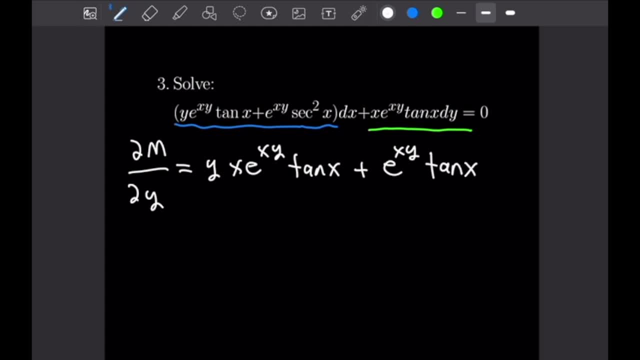 and that takes care of the derivative of our first term there. and then the derivative of our second term is simply going to be x times e to the xy secant squared of x. So let's take the derivative of our m now, so we have the. 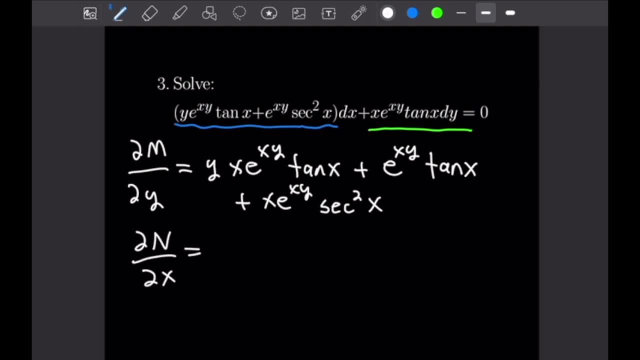 partial of n with respect to x, and that's going to be. let's see, we're gonna have to use the product rule again, but in this case all three of our functions relate to x, so we're gonna have to use a triple product rule, which is basically: 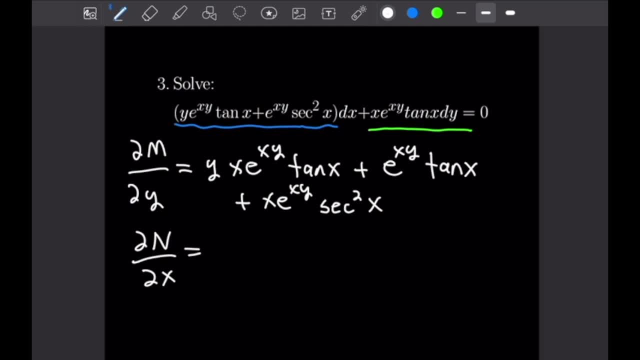 just the same as the product rules you'll see here. So taking the derivative of x will just give us 1, so for our first term we'll have e to the xy tangent of x, and that's going to be plus. let's take the derivative of the second. 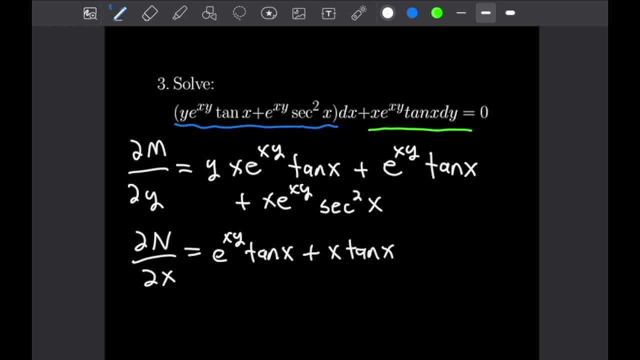 term. so we'll have x times tangent of x times the derivative of that e to the xy, but that's just going to be y times e to the xy, and then we're gonna have plus the derivative of our third term, which is tangent of x, and the derivative of 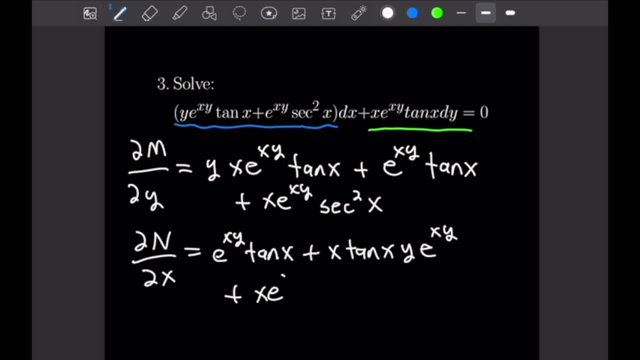 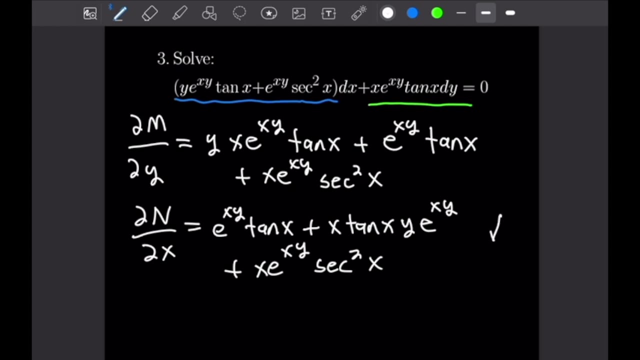 tangent of x is secant squared of x, so we'll have x times e to the xy times secant squared of x, And we can see that that is exactly the same as our dm dy, which means that this equation is in fact exact and we can use our solution method now. Now looking at our m and our n. 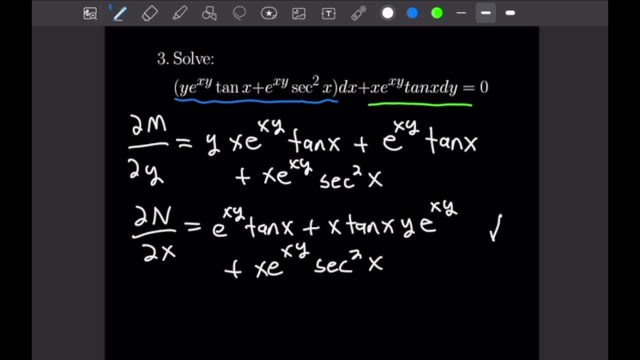 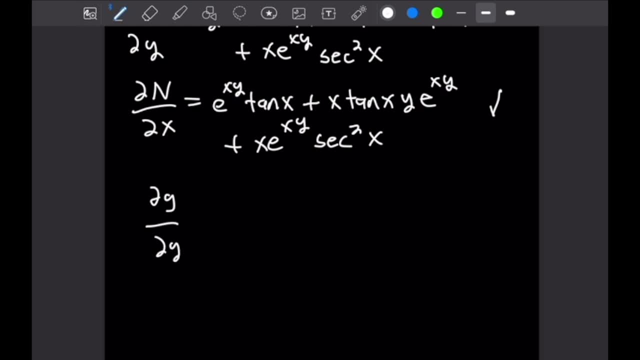 it is evident that it's going to be a lot easier to take the antiderivative of our n than our m, so we're going to use our equation for our m to solve this. So we have that dg dy is equal to x times e, to the xy tangent of x, so we're going to take the antiderivative. 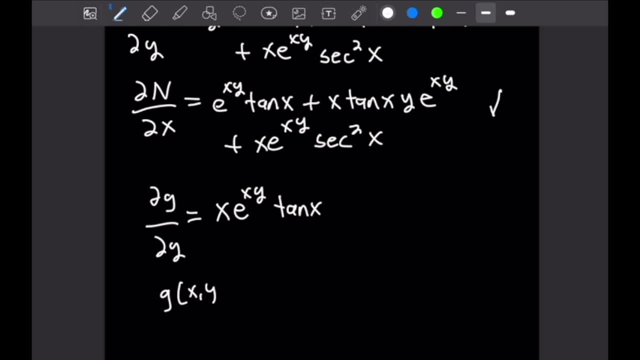 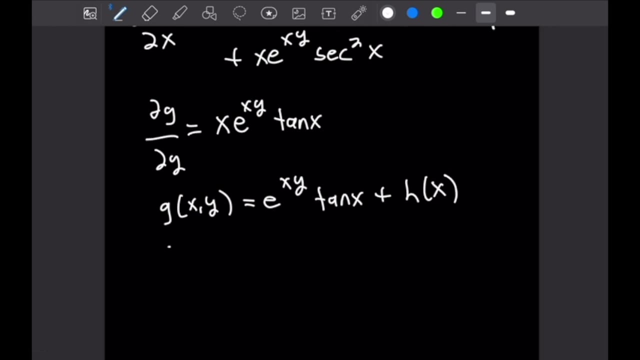 with respect to y, and we'll get that g of xy is going to be equal to e to the xy times the tangent of x, plus some function of x, h of x, And, just like before, we are going to take a derivative to solve for our h of x. so we will get that dg over dx is equal to y times e to the xy times. 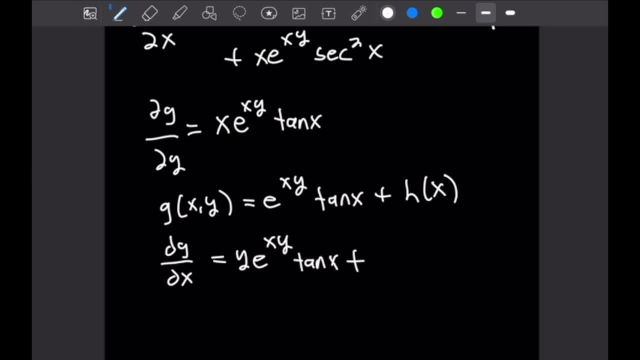 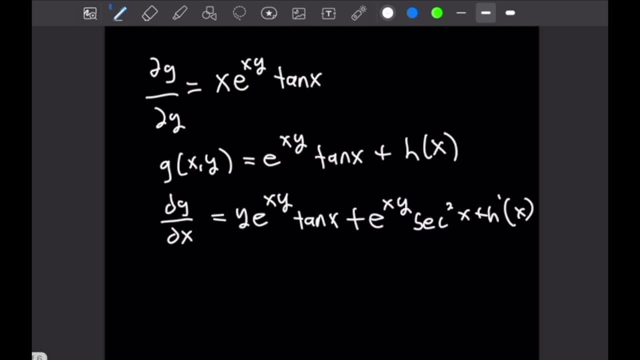 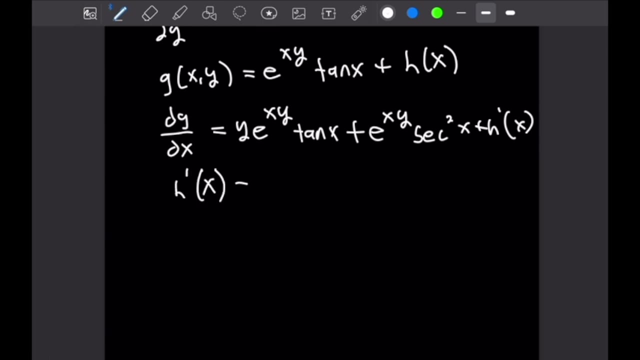 the tangent of x Plus e to the xy times the secant, secant squared of x plus h prime of x, And we can see that that is exactly the same as our m there at the top. So that means our h prime of x is going to be equal to 0, which means that h of x. 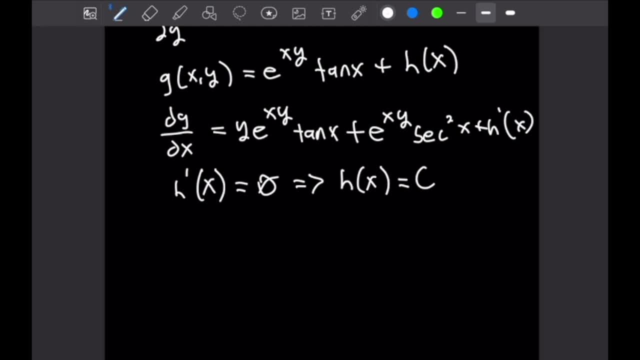 is going to be equal to some constant, which finishes this problem off. We can write our implicit solution as e to the xy times, the tangent of x is equal to some constant, c, which finishes this problem off. So let's get into our fourth and final example. Now for this. 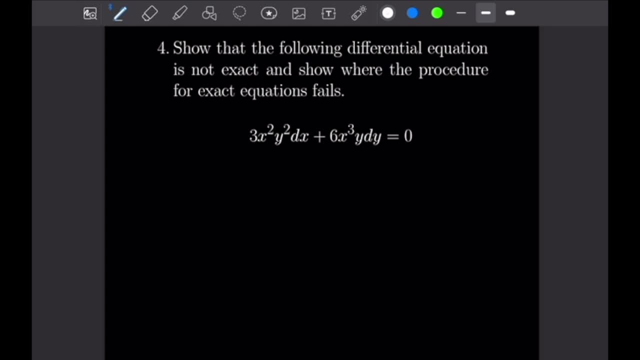 one. we are going to kind of explore why the solution process for exactness fails. So we're going to show that the following differential equation is not exact and we're going to show exactly where the procedure fails for this particular equation. So to show it's not exact.